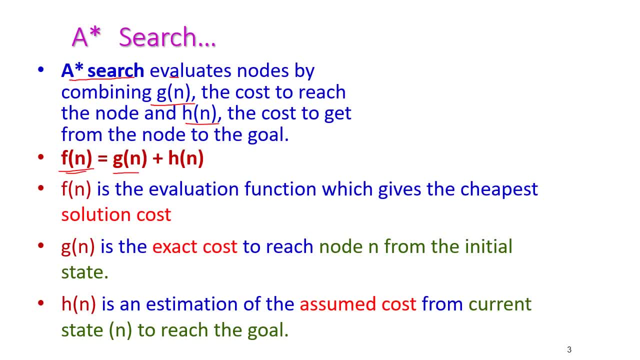 F of n is equal to G of n plus H of n. Here F of n is the evaluation function which gives the cheapest solution cost from starts to goal, Starting state to goal state. So the final solution we will get from this F of n and the G of n is exact cost to reach the node n, that is the current node from the. 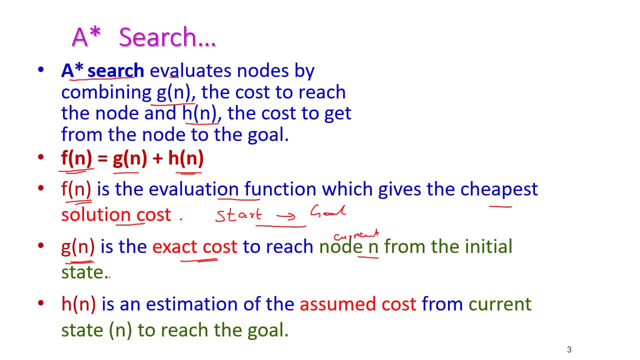 initial state. Okay, So from the initial state to current state, we will get the exact cost. that will use this function. G of n and H of n is an estimation of assumed cost from current state to goal state. Okay, Current state to goal state, we will get the estimation cost by using this H of n- Hence. 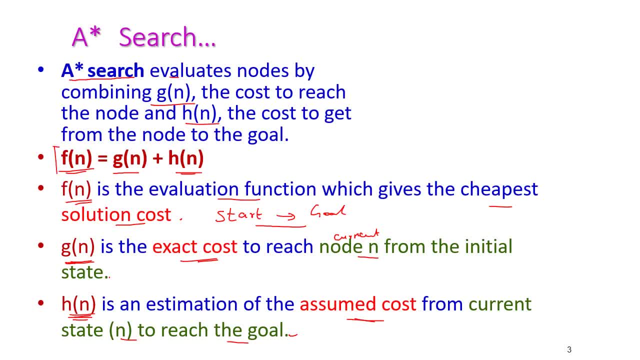 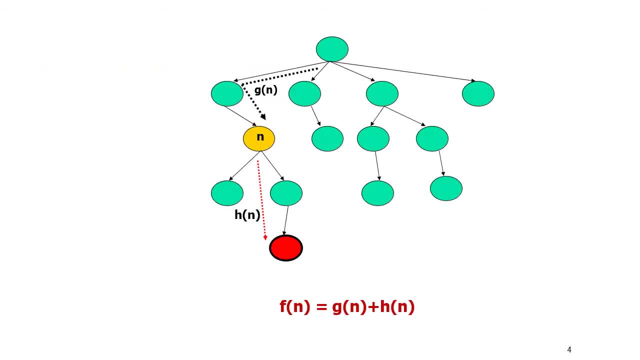 the evaluation function F of n is equal to G of n plus H of n. This is the A-star search. Here. the difference between default state and the defender state is coming from the initial state, So these two values represent the arises and the episodes lost. 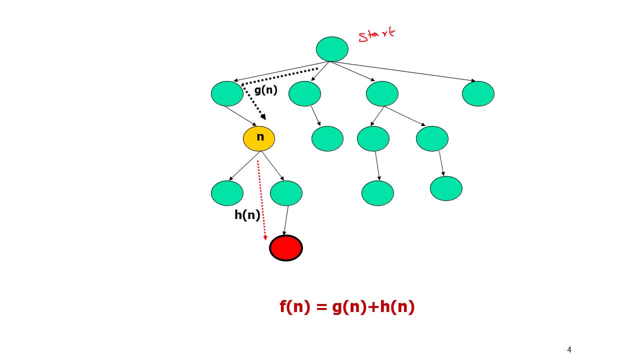 Compared to the original state. we will get G of n there and we will get G of n In terms of verba. we will consider the price of something back. Then our final solution will be a G of n which is D of n. 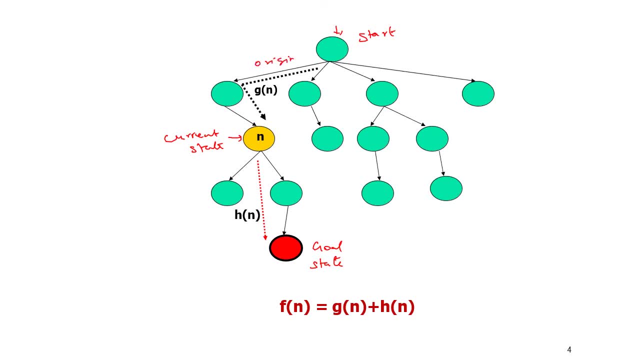 Then the final solution: we will be getting the answer for pulling theback 1.. So first what we will be doing is We will consider fh of n, which is 해. So first, original cast from starting state to this particular state and this state to this particular. 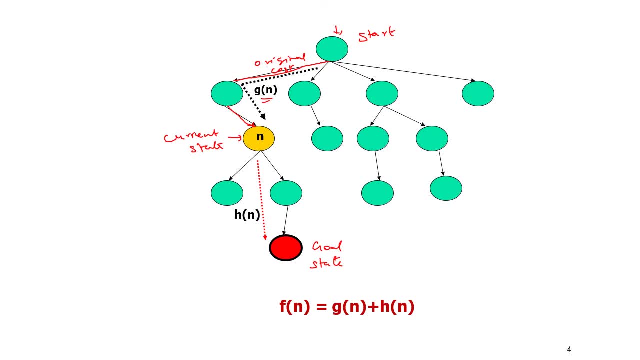 state. okay, so g of n is the original cast of the starting state to goal state and h of n is the assumed cast. h of n is the assumed cast from current state to goal state. okay, for all the nodes, it is having both original cast and assumed cast, right. so the evaluation function f of n is 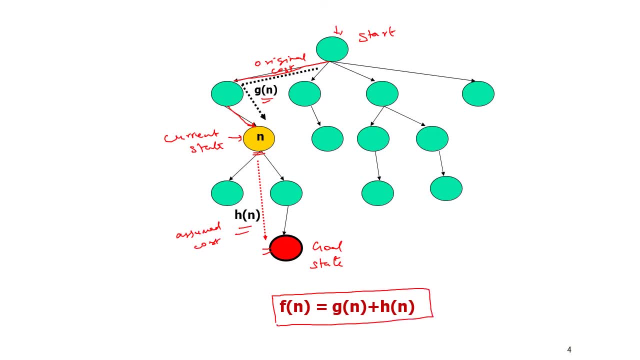 equal to the summation of original cast plus assumed cast. that is, original cast from h of n. is the assumed cast from current state to goal state. okay, so this is the assumption of starting state to current state plus assumed cast from current state to goal state. okay, so this is a star searching algorithm. 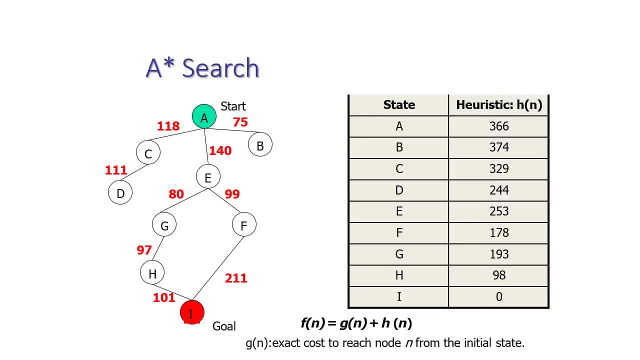 next, let us try to solve one problem by using this, a star searching algorithm. here we need to find the cheapest path from this starting state to goal state, right? so this is our problem graph. so here they gave the cast between two states. okay, so these numbers are original cast. 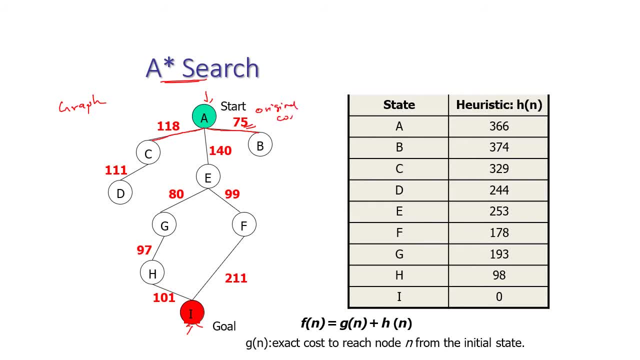 original cast from a to b and this is 118. is original cast from c. a to c and this is 140 is a to e original cast. okay, so in the problem graph they gave the sum. we are described in a mathematical form that according to old. 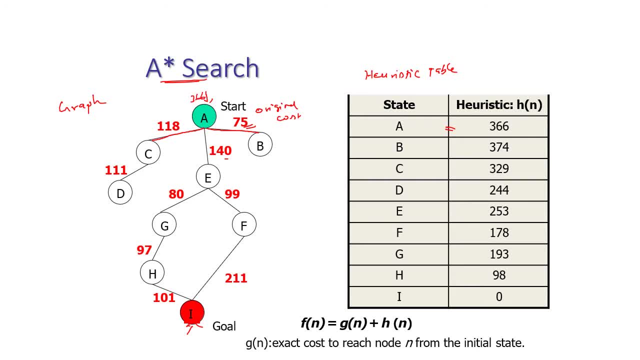 espritie or archaic evolution. okay, so is the algebraic probability is 466 and the assumed cast. and then we divide by 5 or 2�n, which was 3○, and we are given check que Green is equal to c○. 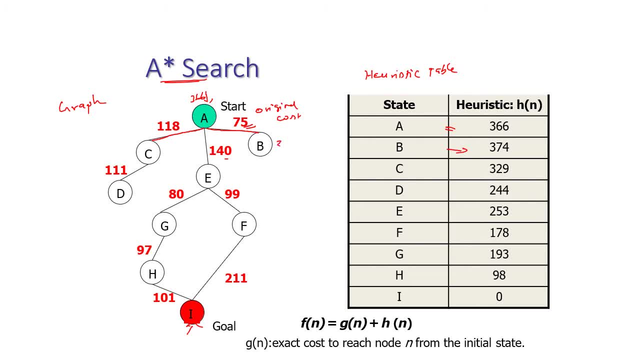 gold, the estimated cost is 374 right, and from c to gold state, the estimated cost is 329. okay, so these are estimated cost. okay. so by using these two value we are going to find the actual path, that is, the shortest path from starting state to gold state. 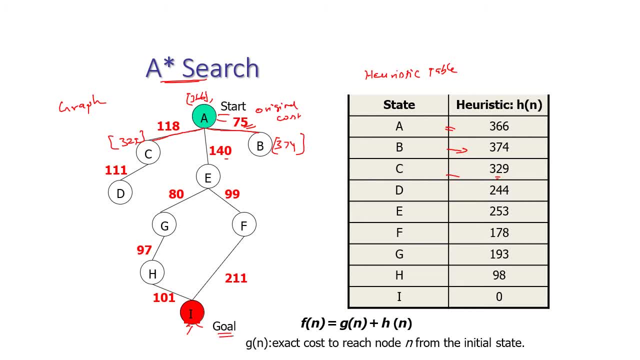 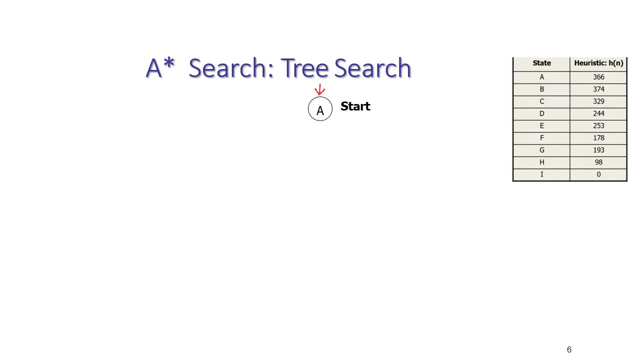 let us try to solve this problem. okay, so our starting state is a. okay, so from a, the heuristic value to reach node i is 366. okay, so we need to expand this a. what are the neighboring nodes of a in our problem we are having? we need to expand the neighboring nodes. so, from our problem we are having, c. 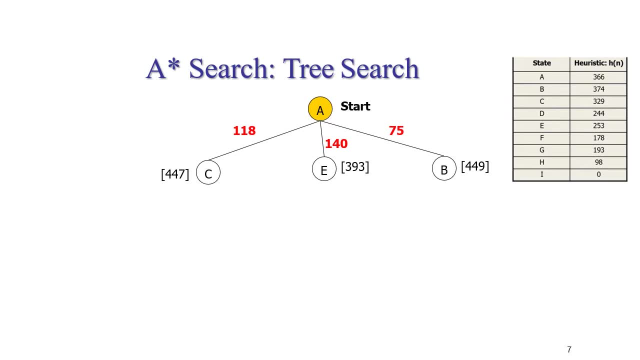 e and b are the neighboring nodes of a, so we need to expand that neighboring nodes. next let us try to compute f of n of c. that is, f of c is equal to g of c plus h of c, right? so what is g of c? g of c is 118 plus h of c. what is h of c? 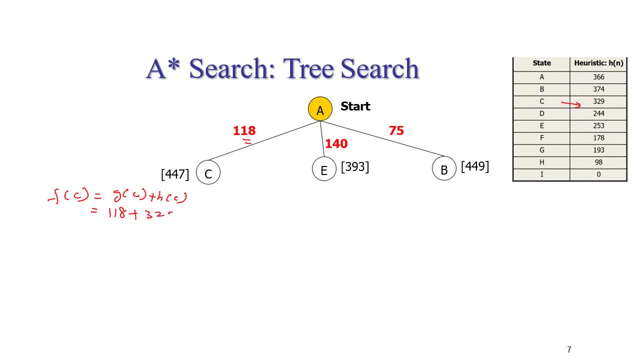 329. 329 is equal to 447. so this 447 is here. also, we need to compute the f of value for all the nodes. okay, next, f of e is equal to g of e plus h of e. what is g of e value? g of e value is 11, sorry, 140 plus h of e value is here 253, okay, 253. so the total is: 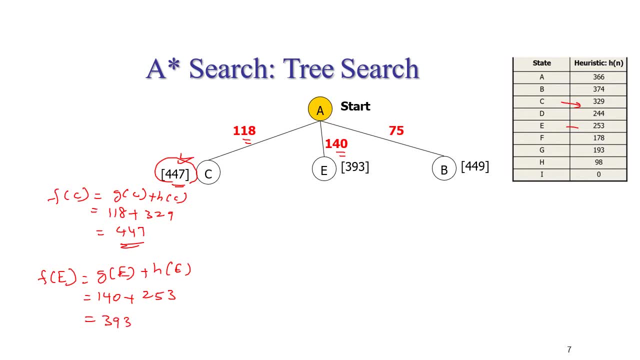 393 and f of b value is equal to g of b plus h of b right. so g of b is 75 and h of b. h of b is 374, 374. what is the total value? 449. that value is given here, so we have to compute. 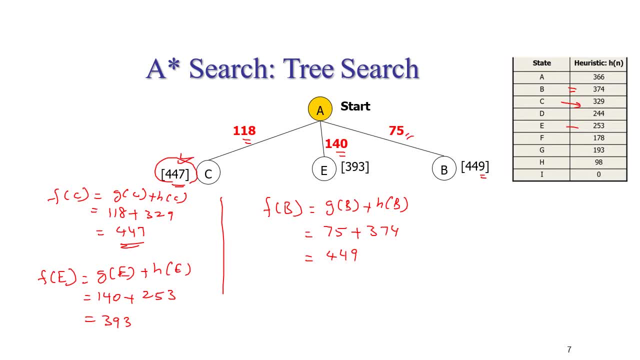 the f of b value is equal to g of b plus h of b right. so g of b is 75 and h of b is 374. so we have to compute the f of value of all the nodes right and next the next step among all these three. 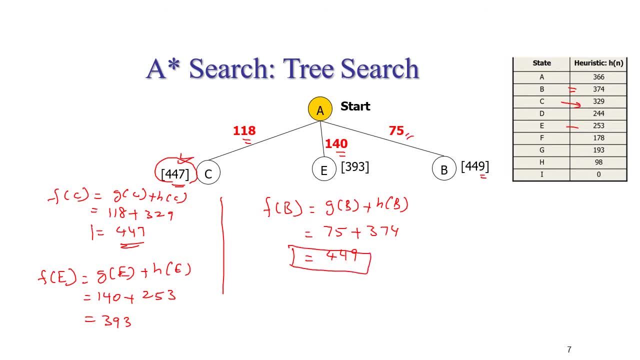 among all these three, which one is the minimum value? f of e is the minimum value, so we have to select only this f of e for expanding further. right, okay, perfect, thank you. so, forнизere, we have to take the 3rd barriers. so we have to take 3rd barriers. 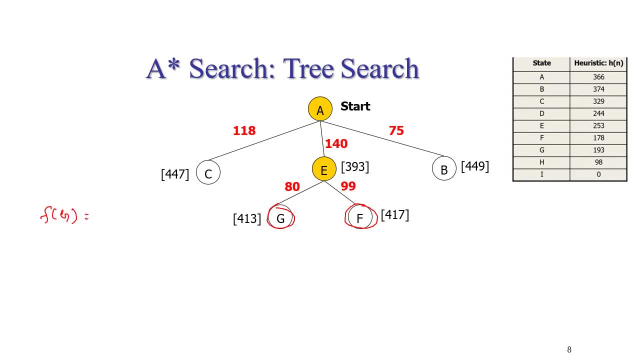 here g plus h, here g minus 1. okay, now we have to write the rest of the values here. we have to write the rest of the values here. we have to write the rest of the values. so for f of e we are having 2 nodes. adjacent nodes are 2 from f of e, so we 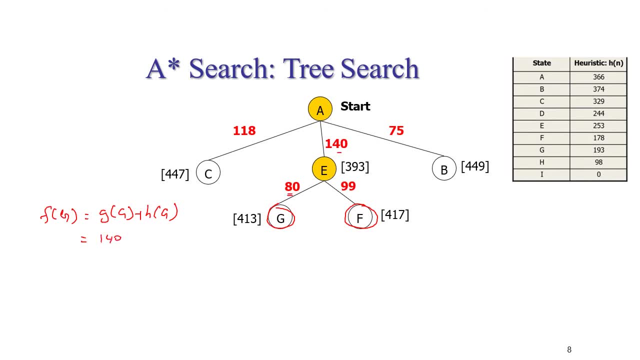 plus 140 right. 140 plus 80 plus h of g: value 193, 193. okay, so total 413 right and f of f is equal to g of f plus h of f. g of f: value 140 plus 99. 140 plus 99 plus what is. 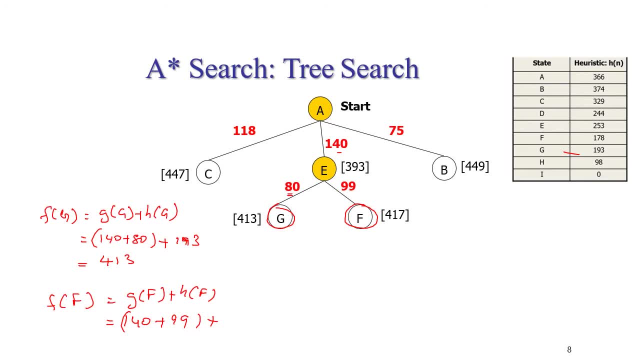 f of f 178, isn't it? so 178, now, what is the value? 417 is the value. okay, so from these two values, which one is the minimum? 1413 is the minimum. so we have to select this particular node to expand further. good, okay. now which is the neighboring node of g, that is h. 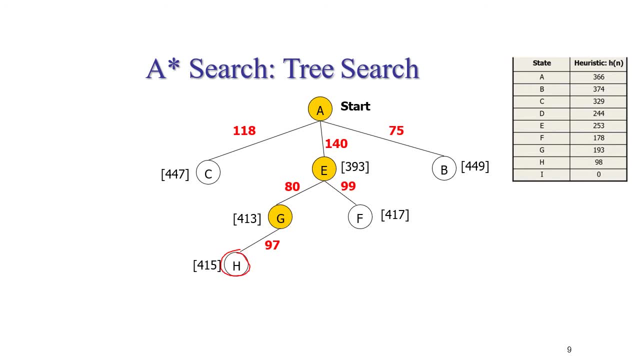 the neighboring node of g is h. next we need to compute the f of h value. f of h is equal to g of h plus h of h. g of h value 140 plus 80 plus 97 plus what is h of h value, that is 98. then the total is 415. right, so from here this is the only option, so we need to. 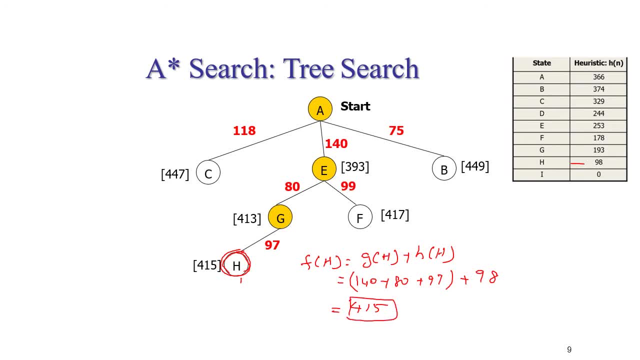 expand the column g z. so we need to expand g z. to figure g z. what is g of h, f of h? then again, we need purple, we need to copy: the prism of will be equal to the number one right. our fold line G z of h is equal to 60. 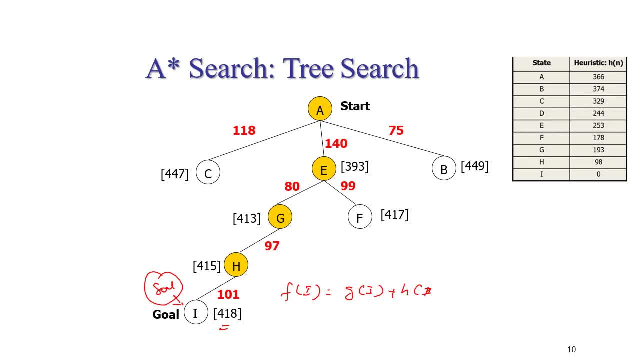 then from here there will be left side. it must be 90 pointzer root or 97 plus 101. okay, what is h of i value plus 0? see, this is the gold node, so there is no need of heuristic value for this. so what is the total? 418 is the actual cast from the starting state to. 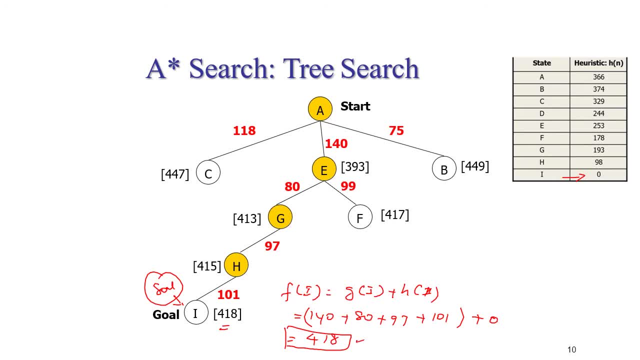 gold state right, and another path is also there. so we have to compute this also from f. we are having i, okay, so the cost is 450, isn't it? so the cost is 450 here. so we have to compute this also from f. we are having i, okay, so the cost is 450. 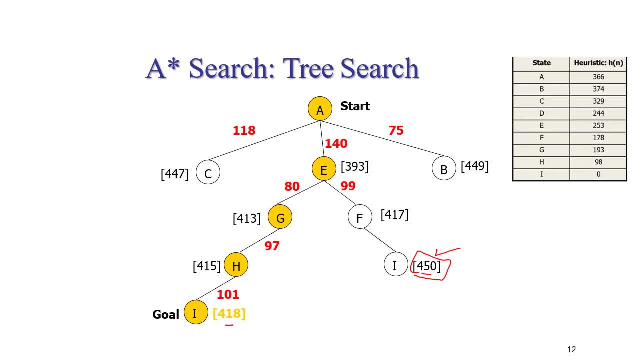 here. so the cost is 450 is very much greater than 418. so this is the original cost. what is the path here? our path is a to e, e to g, g to h, h to i. is the path right path? cost is equal to 140 plus 80 plus. 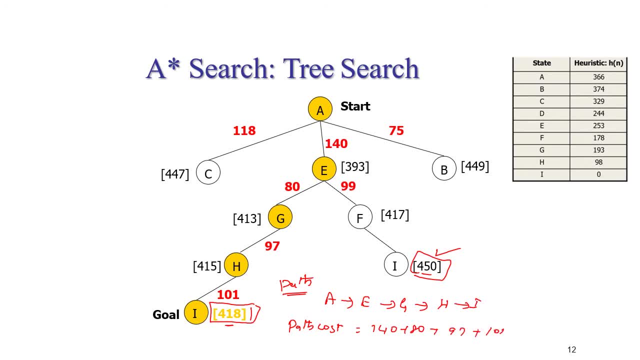 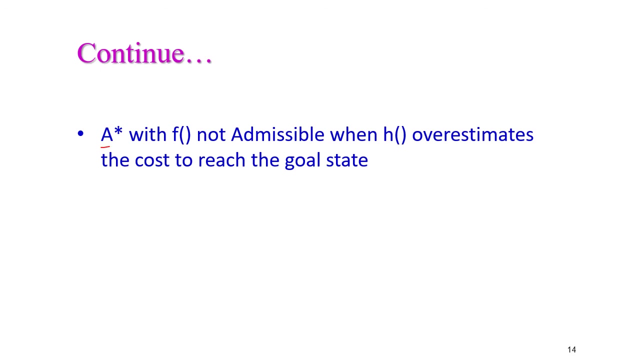 97 plus 101. so this is the path cast. so hence, this is the answer. this is the answer. that is the path by using the a star searching algorithm. right, this is the path and path cast is okay. so a star search with the evaluation function f of n is not admissible. 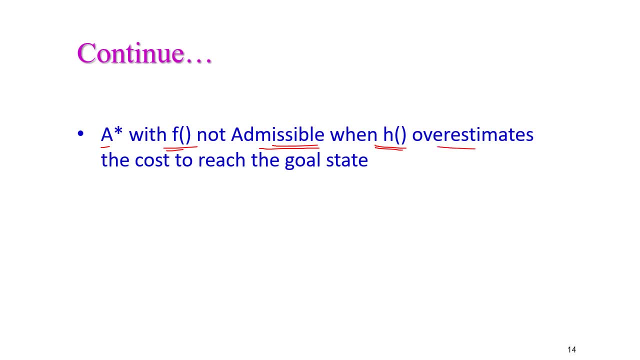 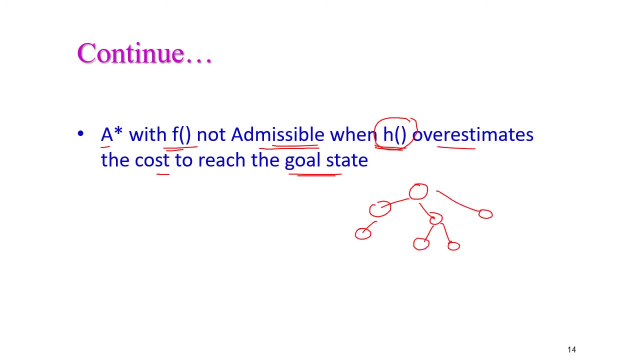 but even though if we look at the, namely the, a star search is letters, get the path, ghost photo, it will not say the path is overstanding 교체, so they shadow, solve the path and we can use this toмоviet then. so much another previous. 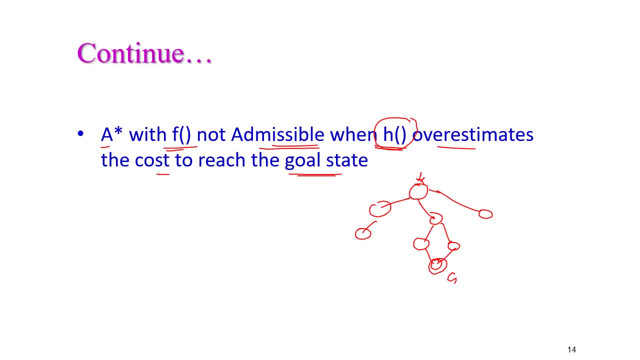 If the heuristic value of here this is A, B, C, D, E, F, G, H, So here the path cast is 2, 4, 6.. The heuristic value of this particular one is to reach the goal state is 10, here 5, this is 20 and this is 30. 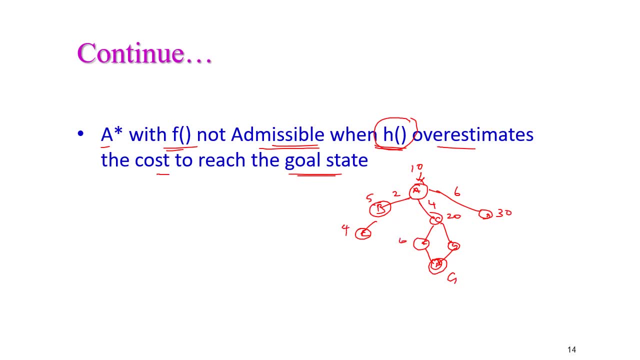 And here 4,, 60 heuristic value. These are all heuristic value. the value which are given in the square bracket, 70, and this is heuristic value, is 0.. So this is 2,, this is 3,, 1,, 5.. 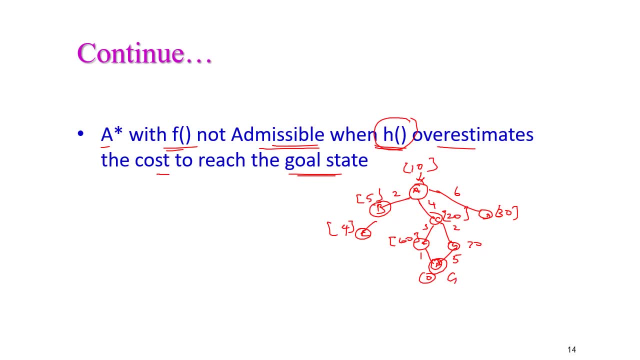 Suppose, if they give such graph means finding the path is somewhat difficult. Why? Because the value given here are: this is 5, this is 20 and this is 30. So the heuristic value is somewhat acceptable. They have to give only the acceptable value. 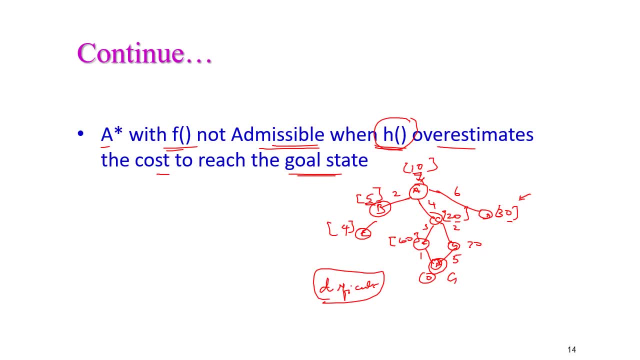 Let me change my pen. If they give the values like this, then we cannot get the value to reach the goal. So the value F should be the heuristic value should be admissible. Then only we can reach the goal. Okay, so this is the problem in A-star searching algorithm. 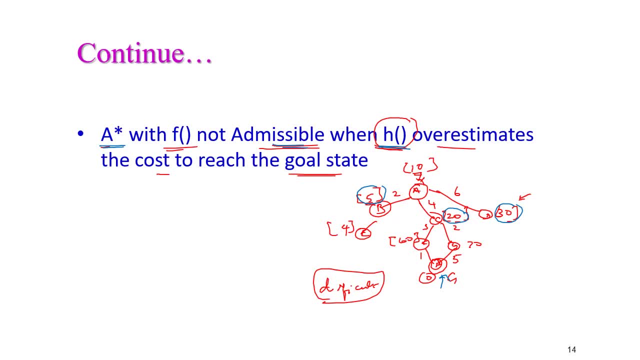 If the value is admissible, then we can reach the goal. Otherwise, it will lead to infinity loop. Okay, so this is A-star searching algorithm. This is actually. this is complete and optimal. Complete and optimal, And up to this we have seen. 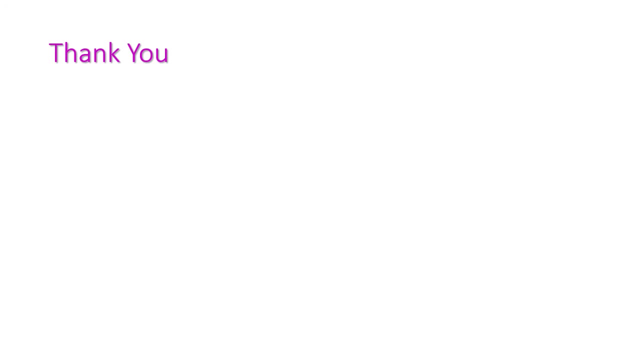 A-star searching algorithm And in the next class we will see the constraint satisfaction problem from first unit. Thank you,